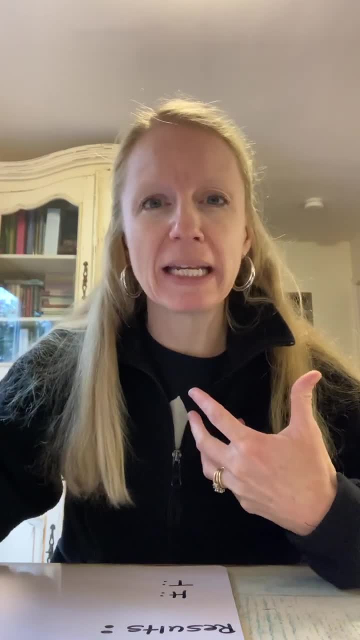 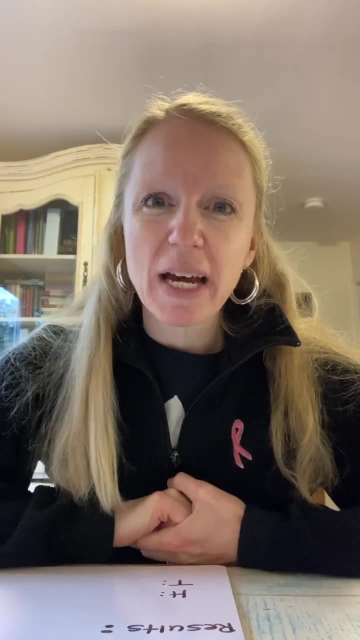 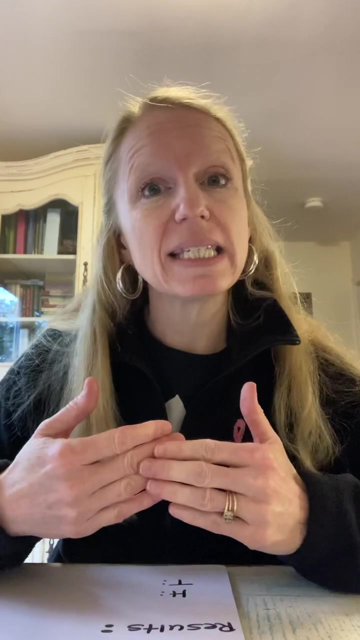 and all of a sudden we have this idea of math probability. And so we say: why are we studying probability? Well, the writers in our curriculum guide helped shed a little light on this and opened my eyes to a bigger concept too. So a lot of things in science can be studied by the scientific. 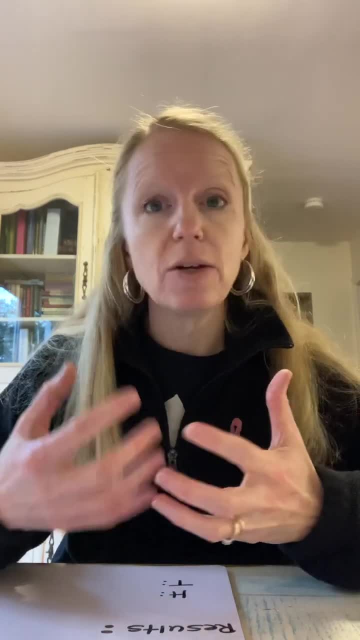 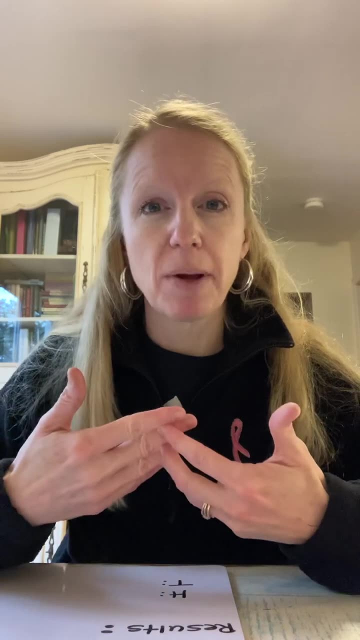 method and by the hands-on little experiments kind of things we've been doing, Of course more complex than what we do, but they can be made into an experiment. However, studies of science such as like the study of origins, are not. 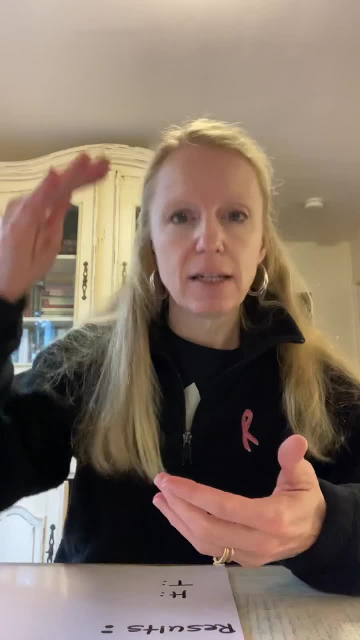 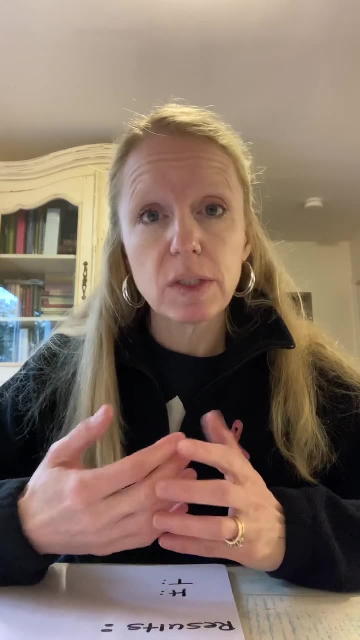 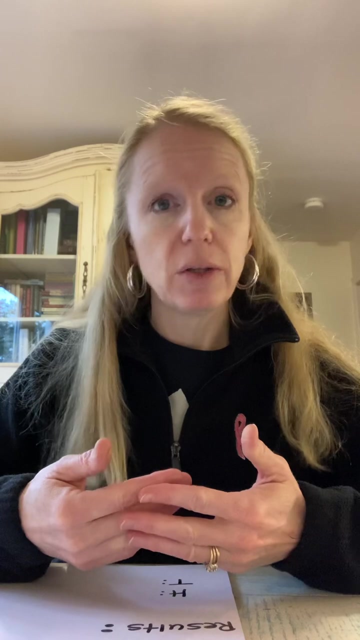 so easily wrapped into a little package and, you know, written out step one, step two for an experiment to be done. In these type of fields, things like probability and statistics are very helpful for determining what's the likelihood that something could happen or could not. just 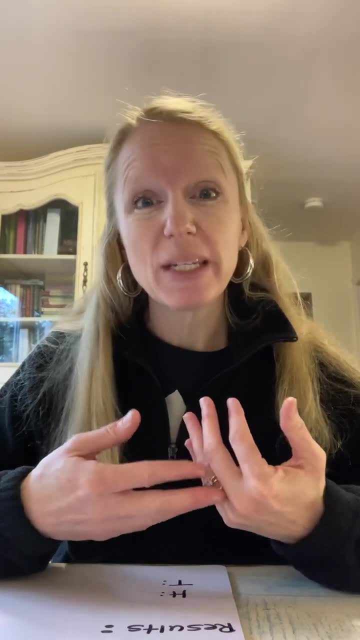 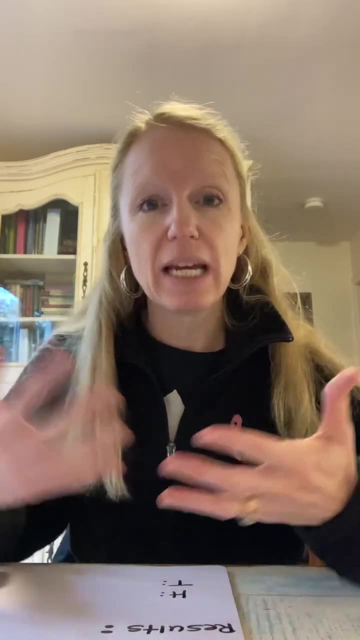 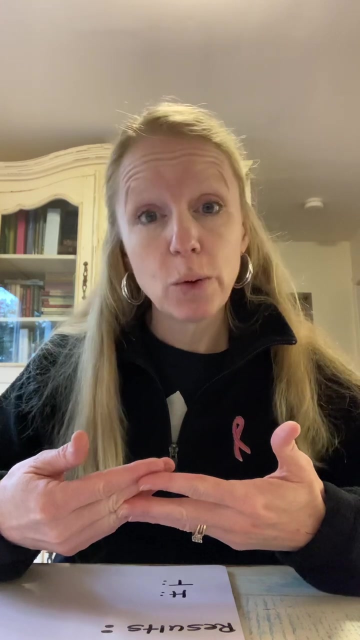 happen, And so for my tutors- and in these little videos you will hear repetition at the beginning of each one- Well, we'll know how itなら enjoy this episode, so they know how important it can be to teach science break right after the meeting and also if you want to learn anything about a thyroid. 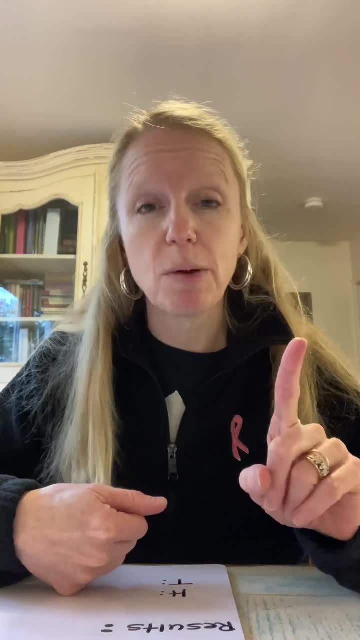 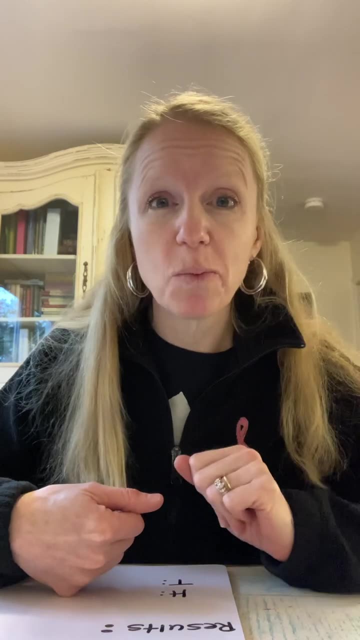 disease, because that is our beauty and health. So let's go. Okay, We're going to take a quick break before we get into the. It's going to take a little bit longer than we actually say, so you don't really need to it. 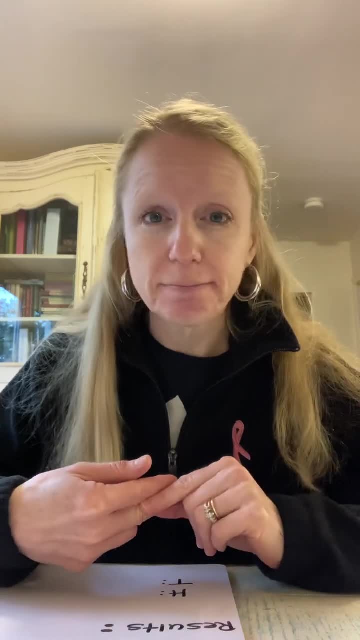 But if you're just cosmic in the seconds of our tail cohort, you are as though you're the most flexible part of gen. än physical is the cool thing that comes and that is also going to be more terrible once it comes. So we're going to learn some things that might interest us and you can correct more than we can. 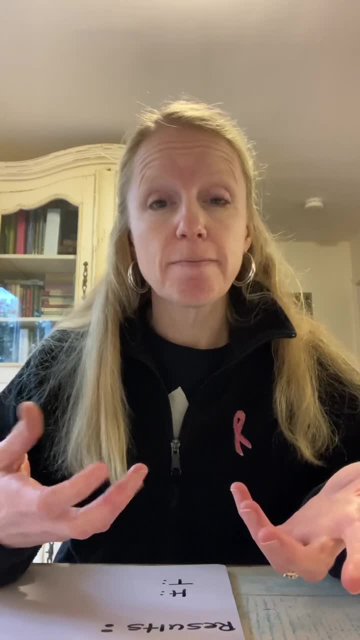 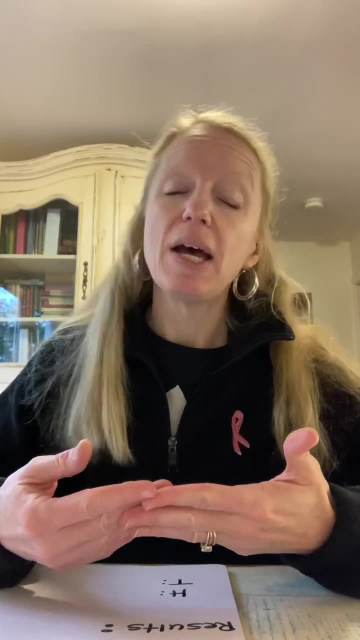 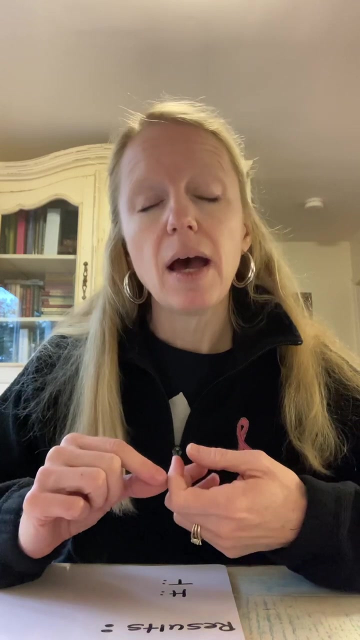 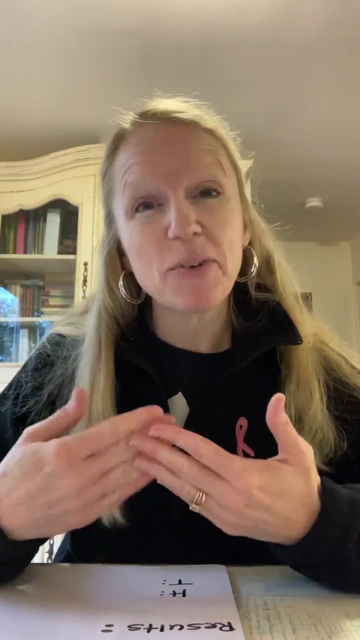 may say, for especially this first week. well, what is chance? well, chance is the possibility that something may or may not happen, and so everything in this life besides God has a degree of chance. everything has a degree of likelihood. it may or may not happen, except for God. Hebrews 13 tells us: 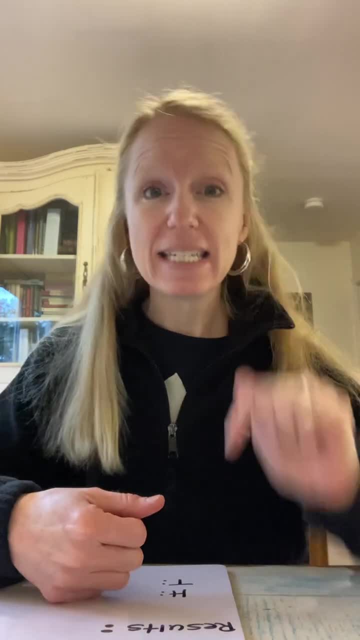 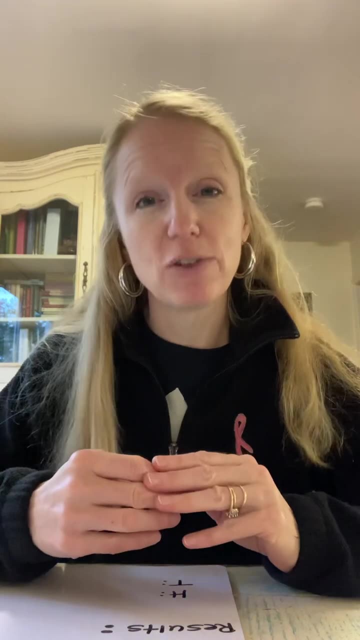 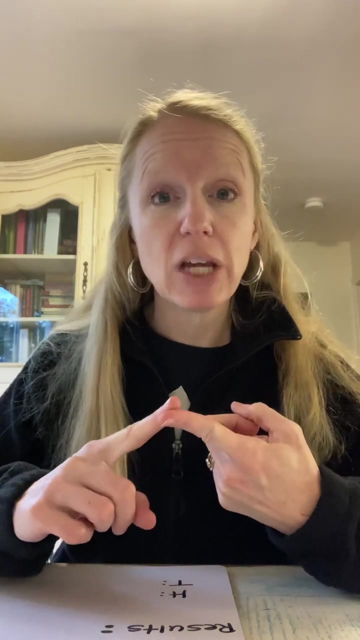 that Jesus Christ is the same yesterday, today and tomorrow, so he is never changing. but everything else has a degree of chance to it. so, with that, that is what we're studying. so probability is the mathematical study of chance. chance, then, is the possibility of something may or may not happen. 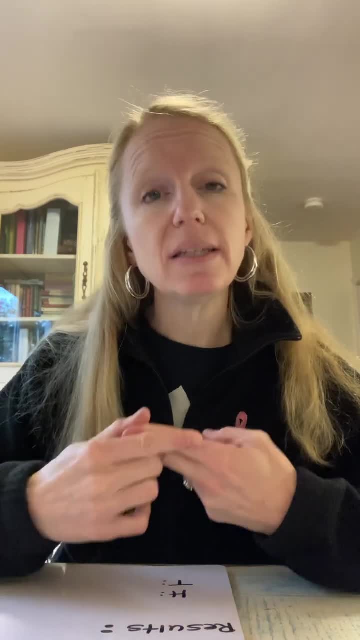 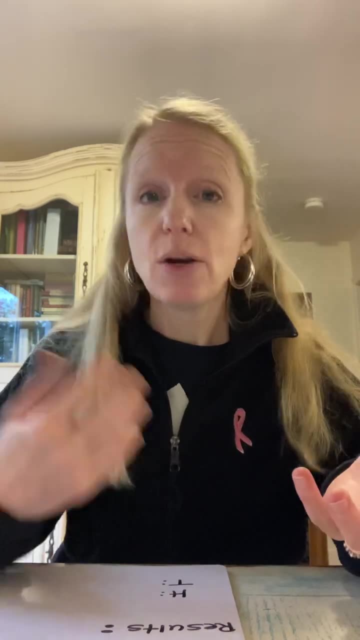 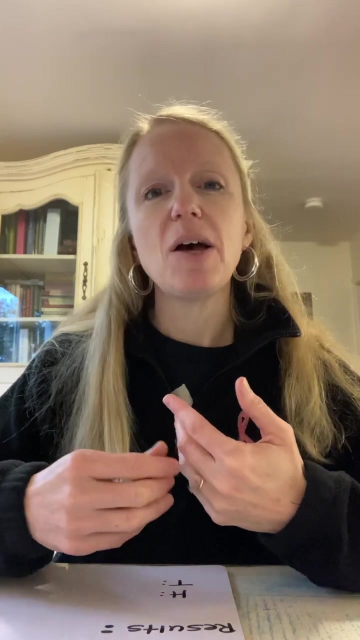 and then why do we study it? we study it so that we can know God's world better, understand why some things could or could not have just happened. there's a book that um Cece used to use. it couldn't have just happened. um talks about the um creation of the world and and looks at 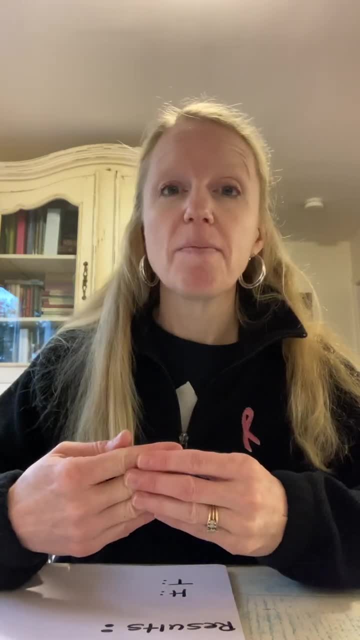 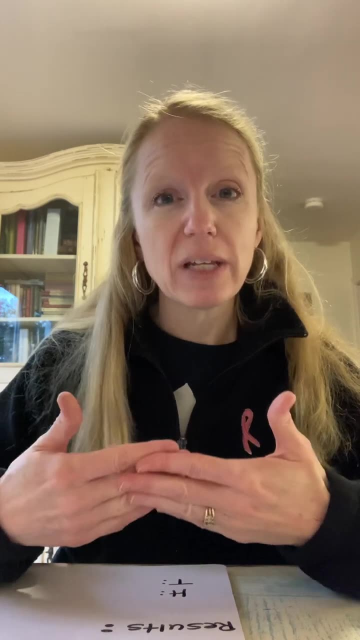 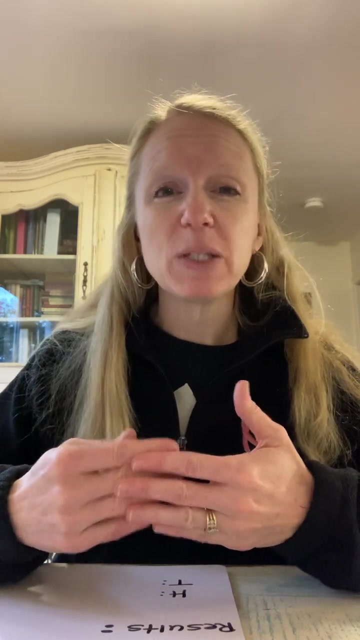 things like that. statistically and probability, um, what's the likelihood that it just kind of happened versus what's the likelihood that our intelligent designer actually has purpose behind everything? um, down to the very bottom line? um, so that is why we study it. it helps us to begin to open our brains to this idea. 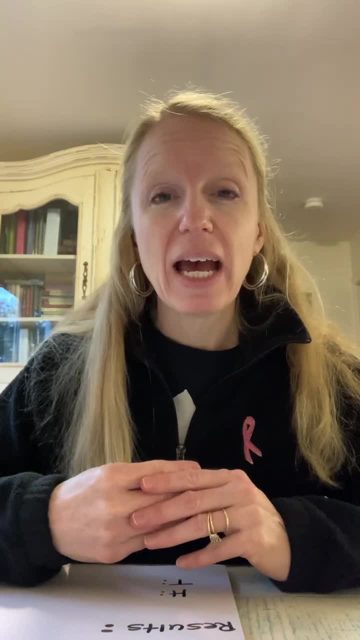 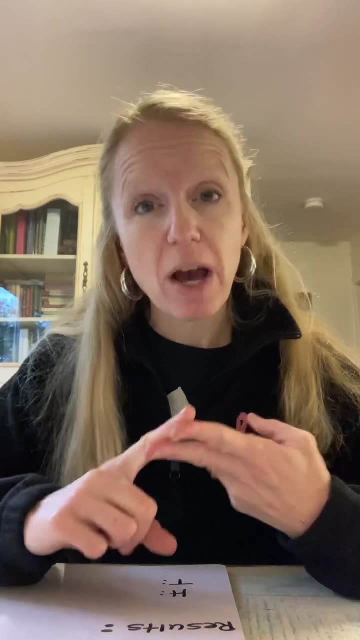 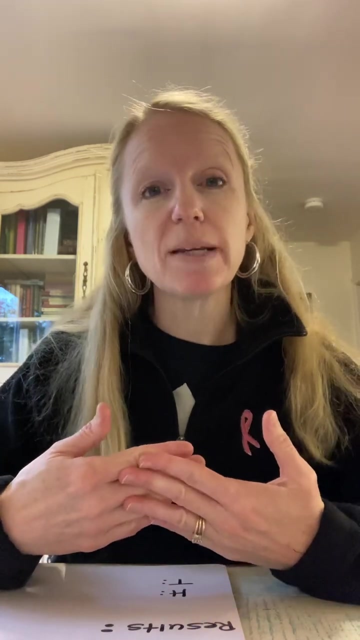 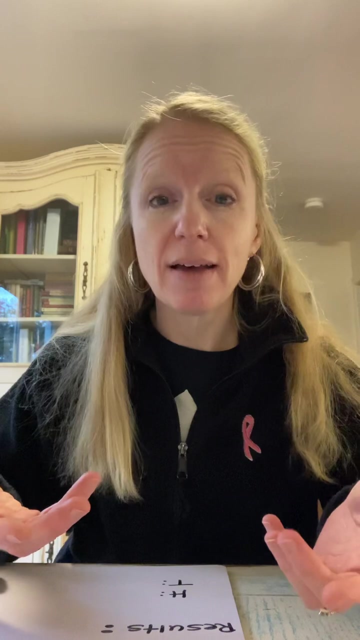 which may, you know, help these kiddos later, um help to understand bigger concepts more so again define probability and why we study it every week at the beginning. so today we're starting with our probability experiments with something called a coin toss. sounds pretty common, um ask the kids, you know, when have they ever done a coin toss? have they ever played that with their 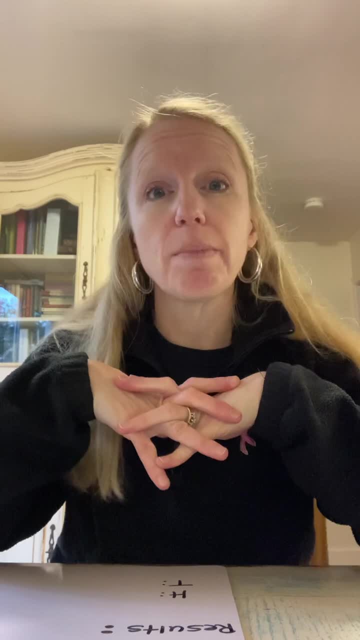 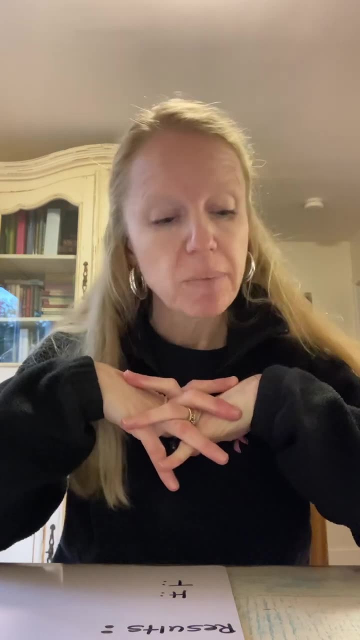 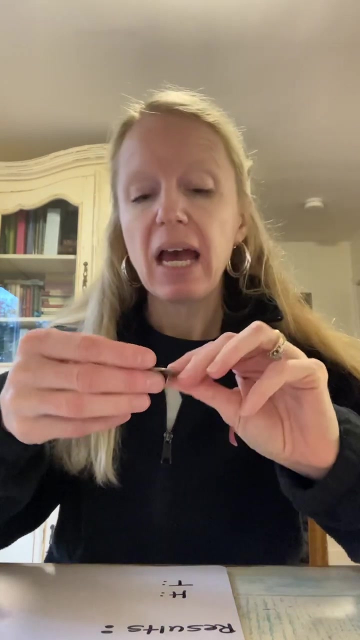 siblings or friends. have they seen it done on the football field or a basketball court? why is it used? what does it mean? because they'll be pretty familiar with that. so a coin toss is simply what it says: tossing of a coin. um and so to begin again, you want to define probability. 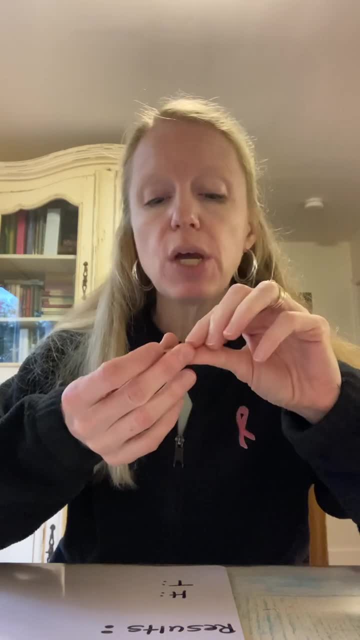 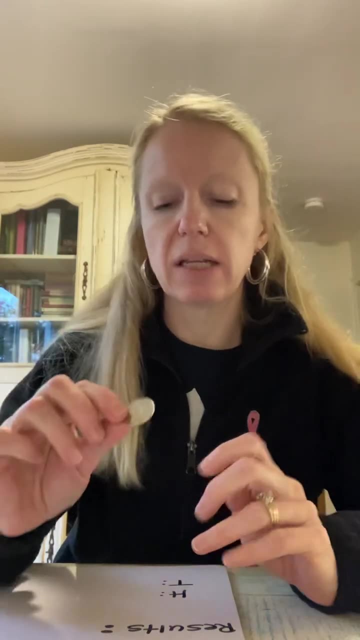 mathematical study of chance. so you want to define probability. mathematical study of chance. so, looking at probability, we want to be able to um write it out so that we begin to understand what that looks like in a concrete fashion. so, looking at our coin, how many sizes this have has two sides. 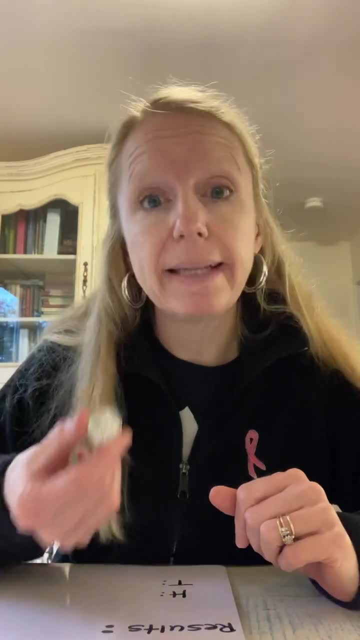 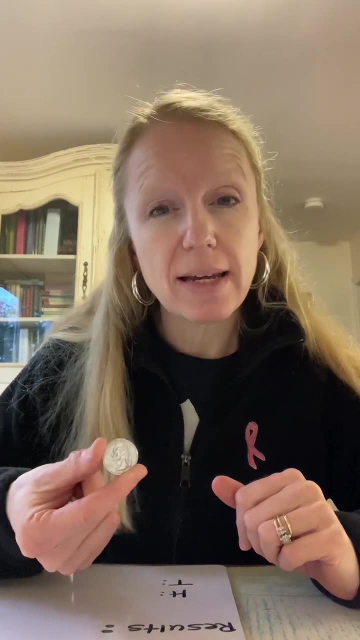 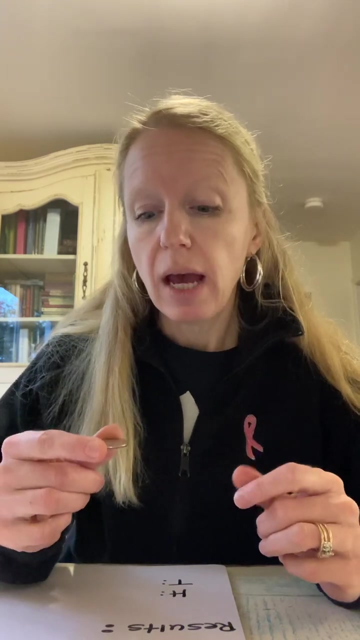 i want to toss my coin and i want a heads up. that is my desire, so i want a heads up. it's always been my favorite anyways. um, so what is the likelihood that i'm going to get a heads up? you might get some random answers. um, probably pretty close fifty percent. um, you know one every. 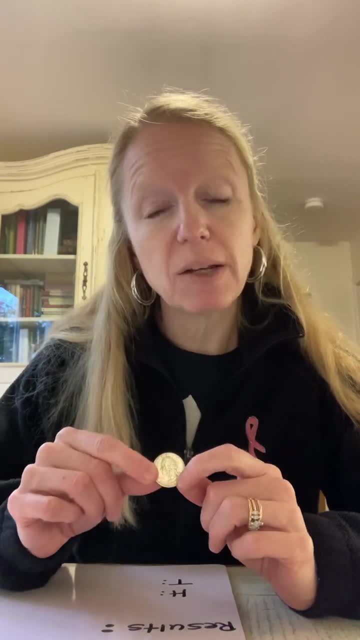 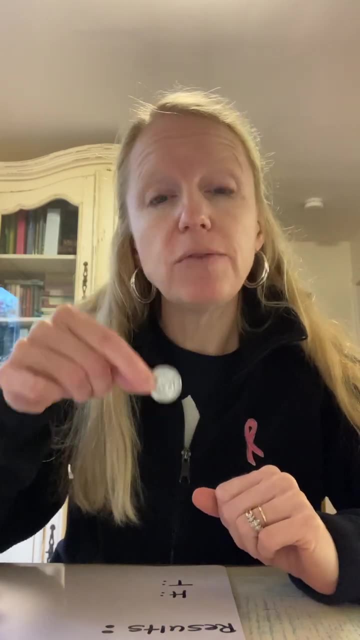 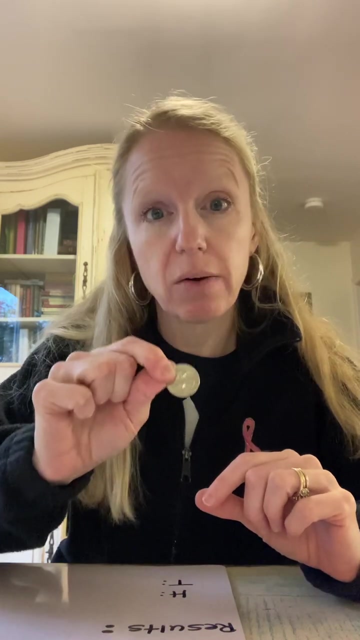 two times um. so to figure this out, probability wise, we write our desired outcome, which would be one. there's only one heads on here out of total possible outcomes, which would be a heads or a tails. so there's two possible outcomes, um, but there's only one desired outcome. so when we write 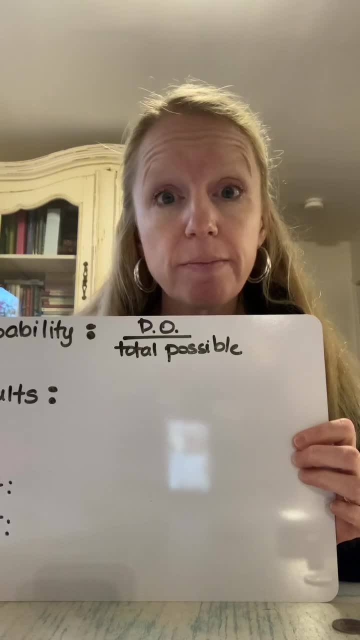 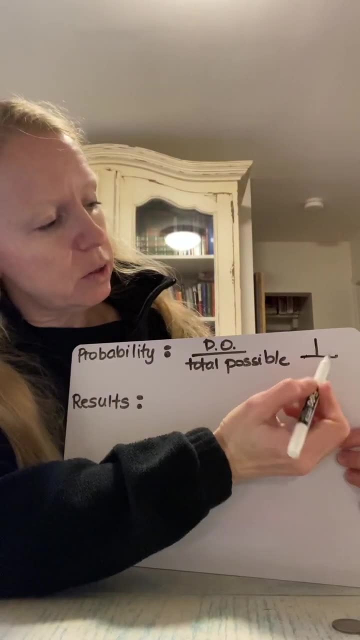 a heads or a tails. we write our desired outcome and we write our desired outcome and we write our probability. We're writing our desired outcome over total possible outcome. So our desired outcome is one. There's only one heads over two out of two, So one out of two chance of getting. 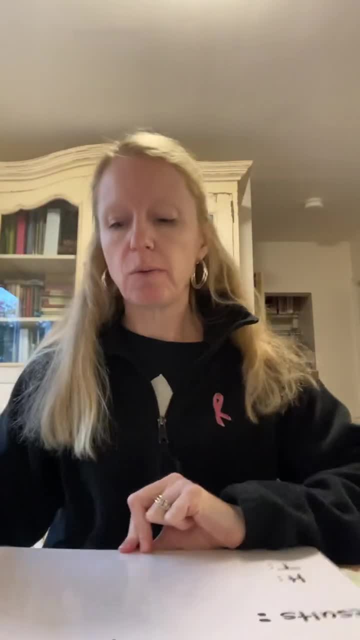 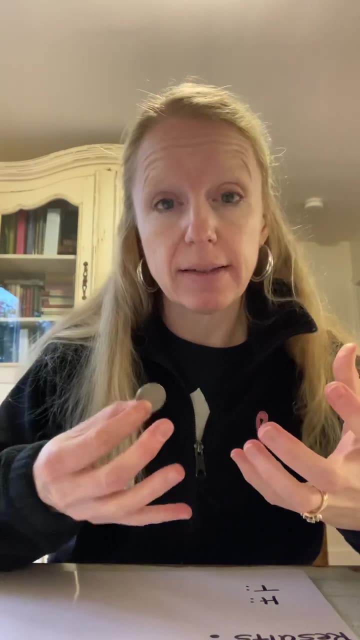 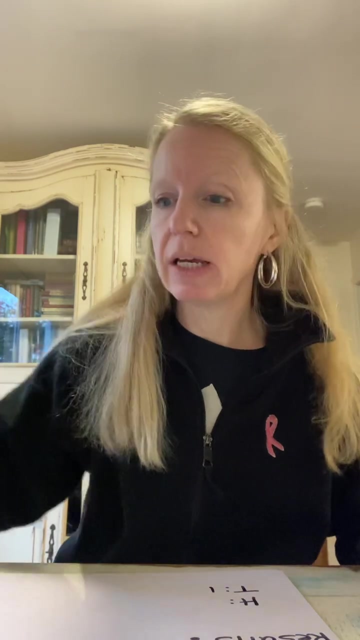 a heads, All right. So we've taught probability, We've showed them how we would write a very basic probability thought, And then we're going to do our first experiment as a class. And so, as a class, you're going to flip this coin 12 times. I'm going to do it very quickly here, just so I can. 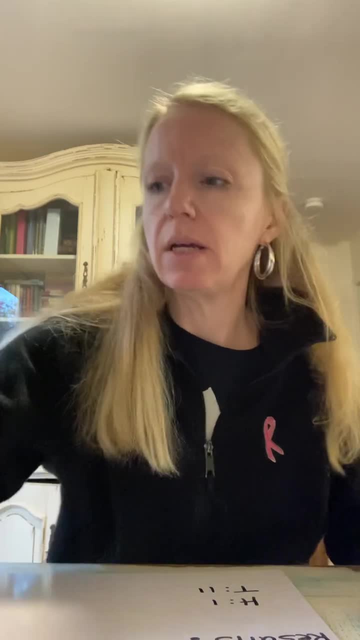 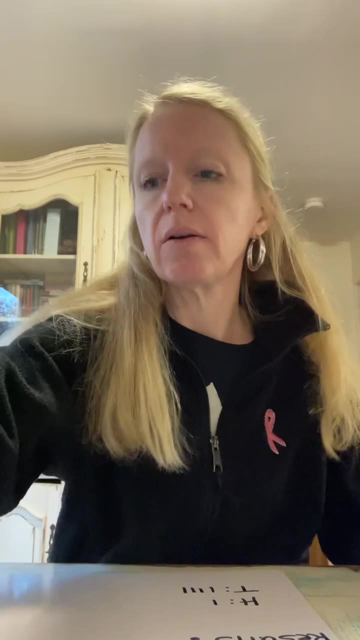 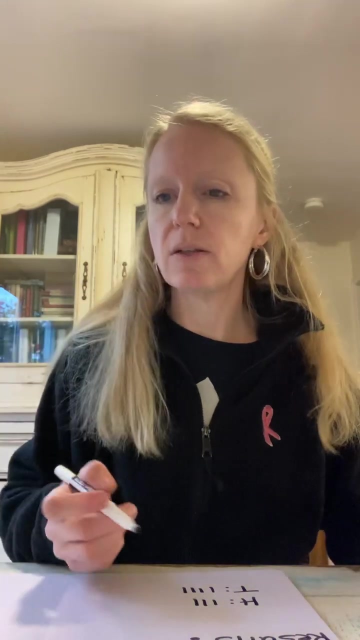 show you. I got two heads here, One tail one. oops, sorry, there's a heads and a tails. Let's say: I keep going here And I get all. right, now heads are winning Once you do it 12 times. 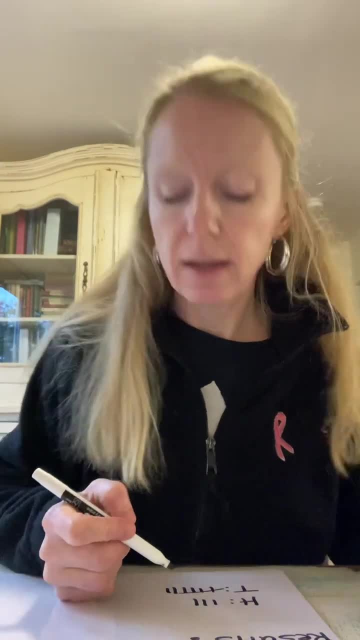 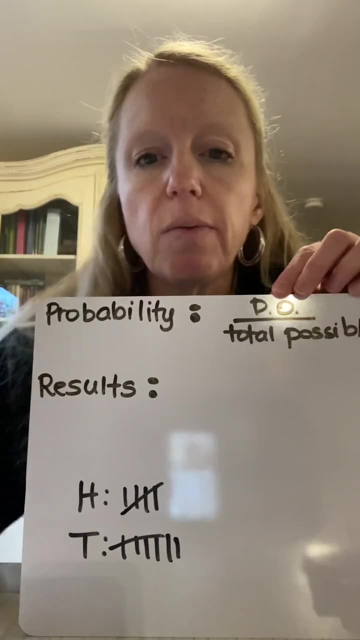 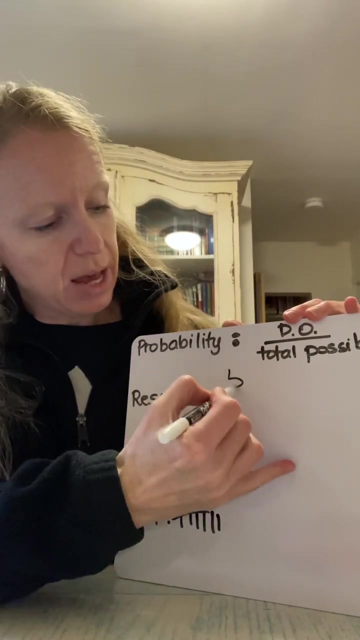 oh gosh, I got a lot of tails here going. I got a heads, All right. So let's say we did 12 times here And my results were five heads and seven tails. Okay, So my results were five heads. 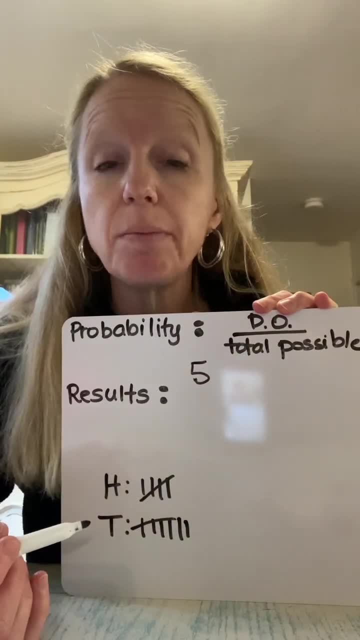 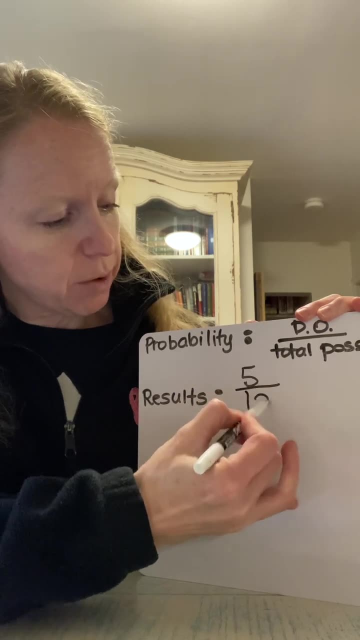 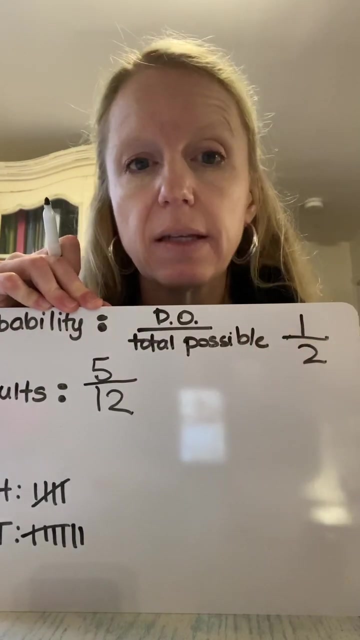 Okay, I got five heads right Out. of how many possible times did I toss it? 12.? So my results were five out of 12.. Okay, So results as you can see. so if we were to make this a, you know, a smaller fraction, 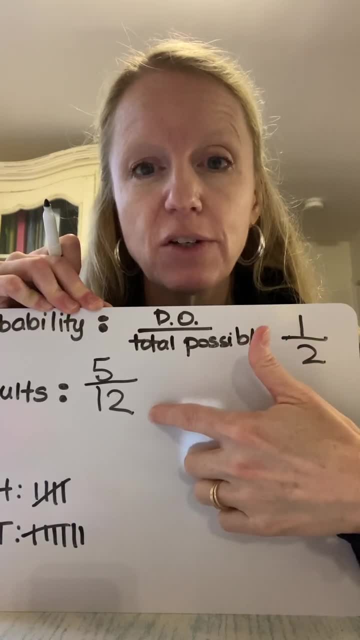 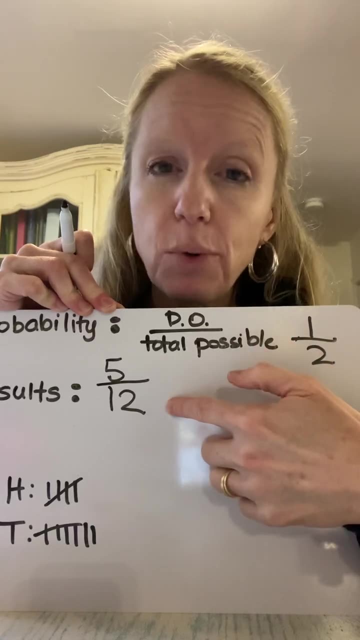 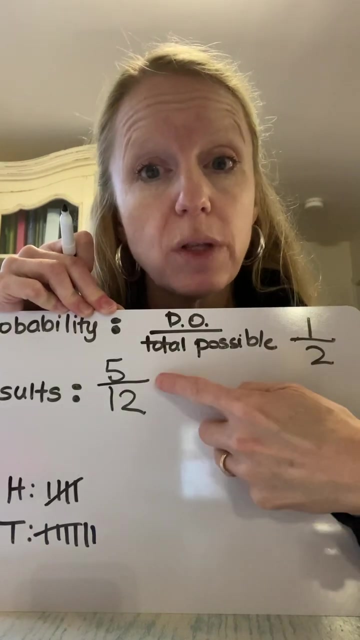 it would turn into not a perfect fraction, So I'm not going to do that, but we're actually pretty close to one out of two, one half. So results- this is important- Do not always equal the probability, But usually the more results you do, the more data points you have, the closer you get. 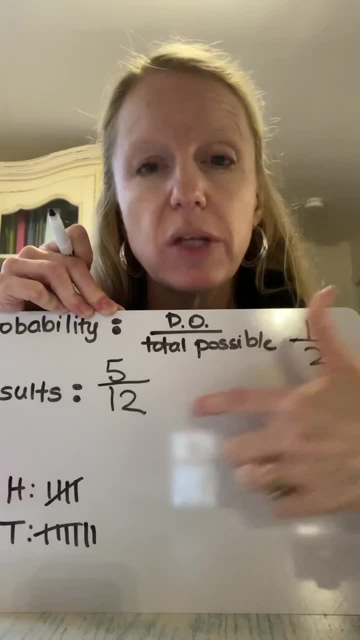 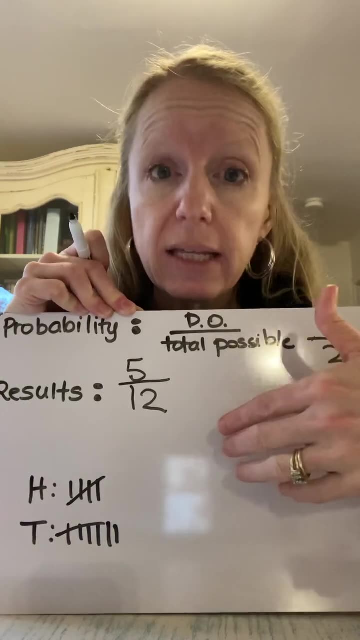 to the probability of something happening to them equaling or being really close- which mine was really close, just with 12 tries. And so you want to show the kids the difference? There is a difference between results and probability Because, again, probability is. 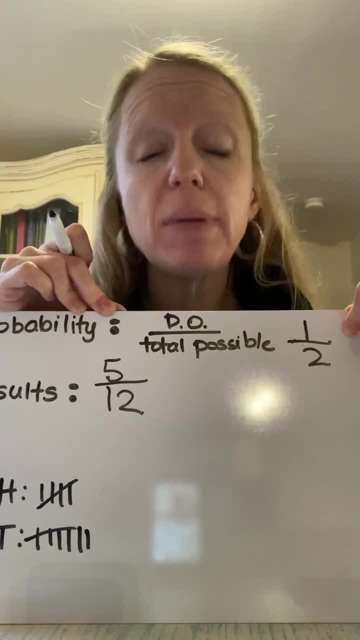 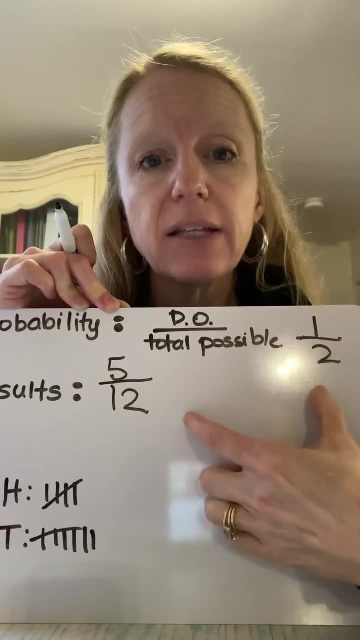 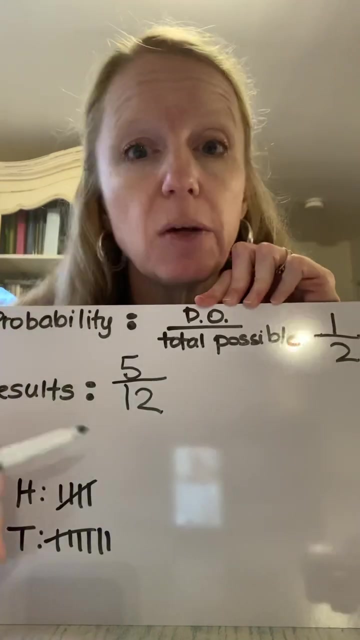 the study of chance. It's just the chance it will happen. It doesn't mean it actually will happen that way, but it's the likelihood that it will happen. And again, that gets closer. the more times you do that gap, It gets closer. If you wanted to turn it into percents, you would then just divide these You. 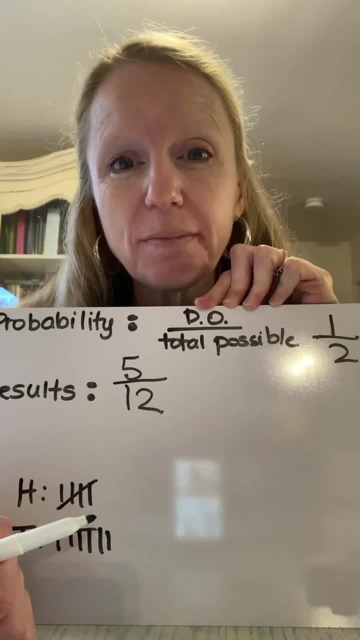 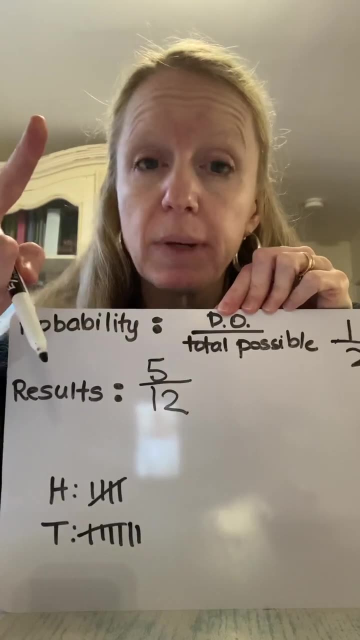 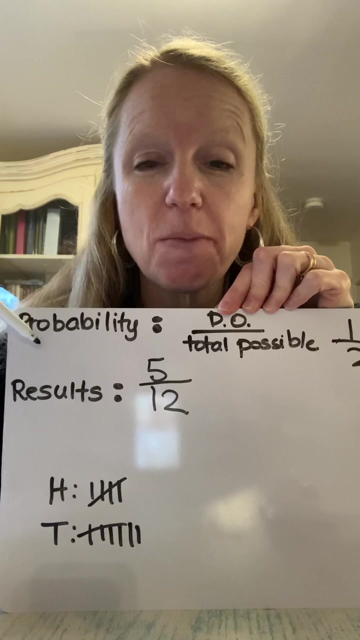 can use your calculator and then multiply times a hundred and you would get pretty close to 50%. So that's so. again, we're defining probability, We talk about why we do our coin toss as a group, And then we talk about the difference between probability and our results. 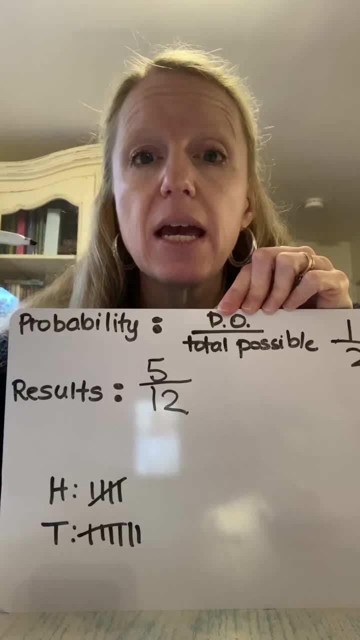 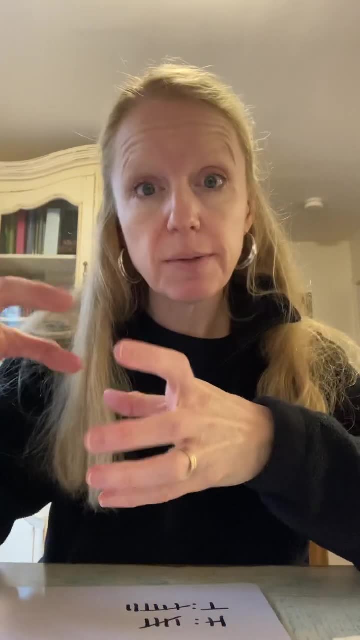 because that will be something you look at every single week, And then you're going to do a little bit of math. So you're going to do a little bit of math, You're going to do one of two things. You're going to rather break off into stations, three stations. 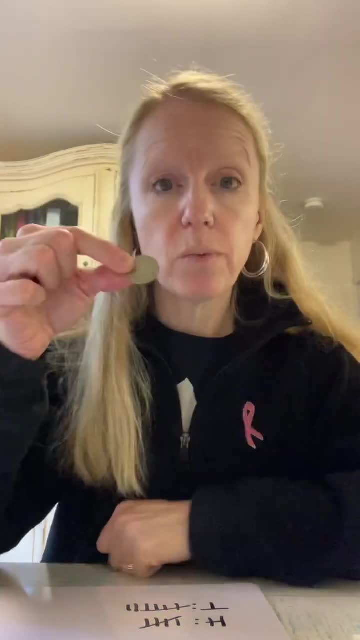 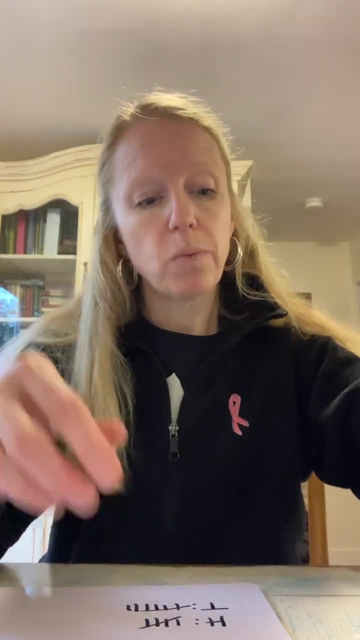 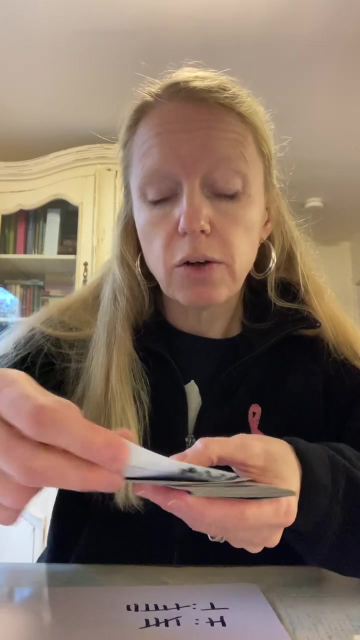 One will be, at least in my campus. we'll have one coin toss station. We're going to do exactly what we just did again and calculate their results. We're going to have one card station where kids will each take a turn. They'll pick 12 cards and you're going to be documenting if you got a black or a red. 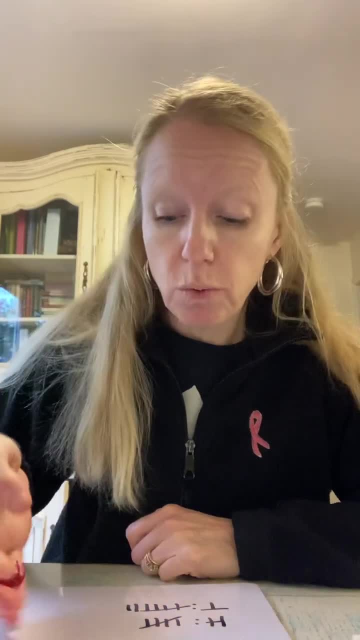 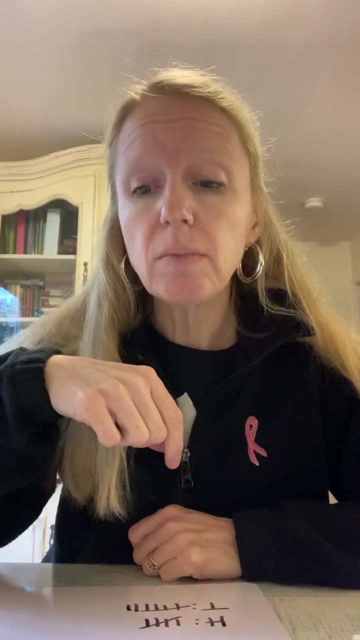 The third station will be a dice station Where they'll roll their dice and they'll keep track on the charts. I'm going to show you in just a second of what number they roll. You have each set of three kids at three stations. 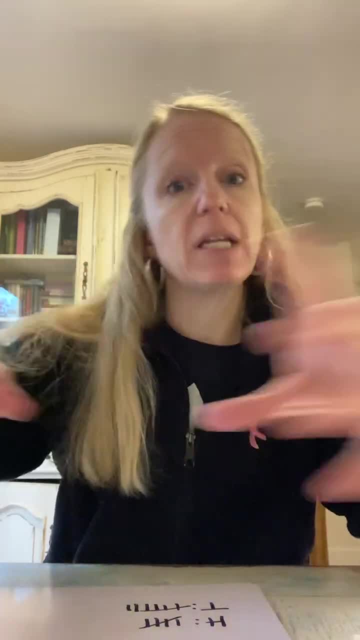 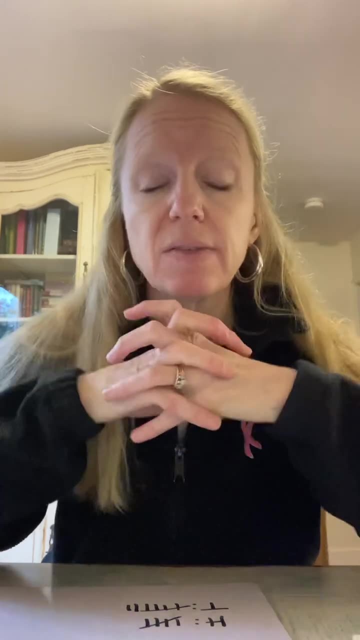 After five minutes shift stations. After five minutes shift, again and again. So you spend about 15 minutes doing these different experiments and getting the results And then spend the last five minutes of your class going over the results as a whole. We will do a little bit of math.